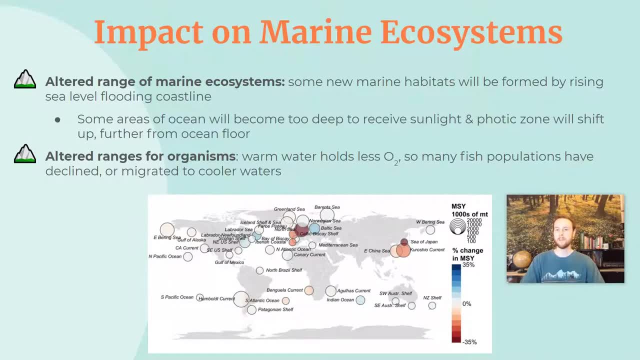 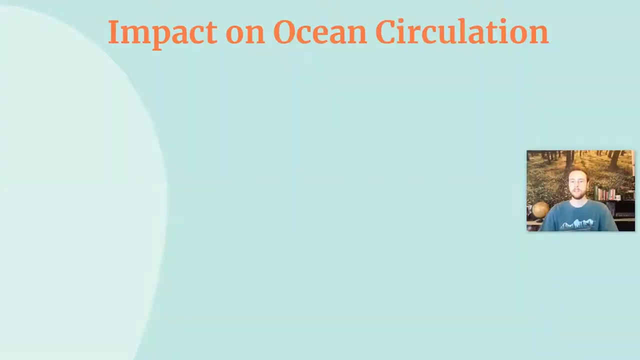 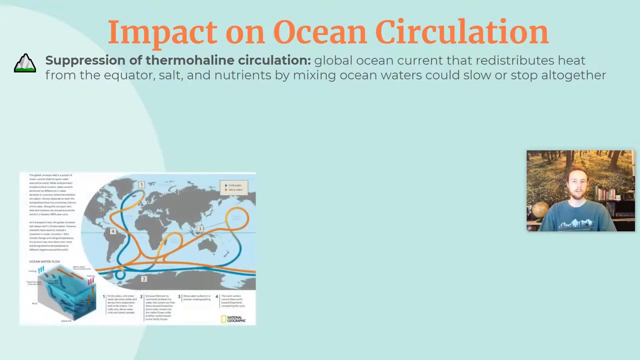 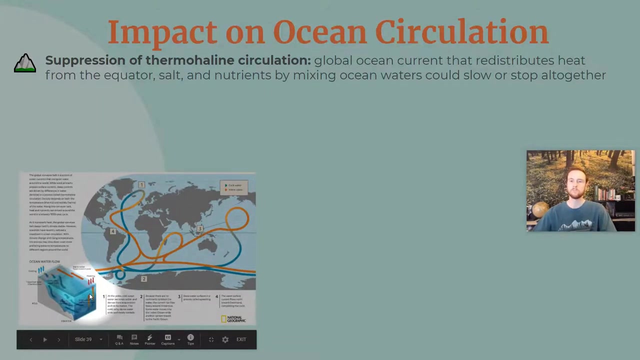 And so, we can see that the maximum sustainable yield, MSY, which refers to how many fish can be caught sustainably without causing collapse of the fishery. That's going to go down for many different species of fish in many different parts of the world. And again, that's because these fish populations are either becoming smaller, as many of their members are killed off, as water warms, and we have less oxygen. Or many fish become less active. Or we have less marine habitat, and those like that, they are more protected, so they are less susceptible to water and in the water or they're migrating elsewhere they may have to go see colder waters in order to get those oxygen levels that they are adapted to now we'll take a look at the impact of climate change on the thermal haline circulation or oceanic currents so remember from unit 4 that the thermal haline circulation is this global pattern of warm equatorial waters expanding and moving away from the equator and carrying some of that heat in the atmosphere and in the ocean out towards the poles and so if we take a look at this national geographic diagram here this can be really helpful for us understanding this in a little more depth so we have this cross section here which is really helpful because the 2d maps make it hard to visualize what's really happening and so we have the equator on the right hand side of this kind of cube view and we have we'll just call it the north pole on the left hand side and so at the water's level here remember that the sun's rays are going 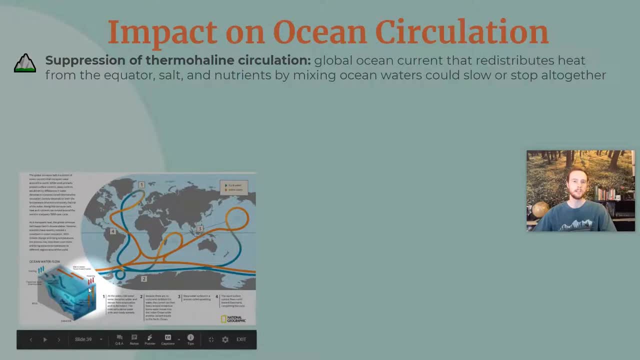 to be most direct and so this is going to be the warmest water that water is going to expand and spread out and it's going to spread out and it's going to spread out and it's going to spread out towards the poles and if we follow along on the 2d diagram we'd be moving here and then you know you get the gulf stream which is this mass of water redirected from the north american continent continuing up to the north atlantic up towards the poles now when that warm surface water reaches the poles it cools down also because a lot of it has evaporated on the way it's going to be a little bit more salty than it was the salt's going to be more concentrated and so that cold and salty water is going to be more dense and so it's going to sink and that's really important because when it sinks it goes down to the ocean floor and it mixes nutrients and salt and other things that are dissolved into the ocean all throughout the ocean floor and then eventually it will rise back up to the equator and so it redistributes heat it redistributes nutrients and oxygen and many people refer to it as the ocean's conveyor belt or the earth's conveyor belt and so it's a very critical process on earth for distributing again heat nutrients oxygen very important to earth's climate so now if we look at what's predicted to happen with climate 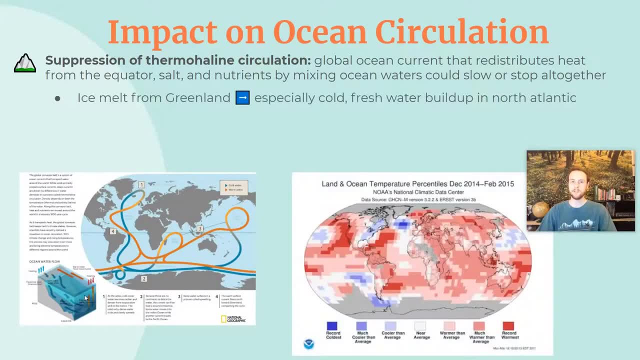 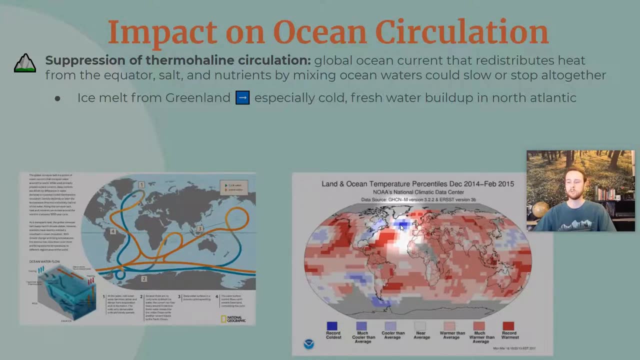 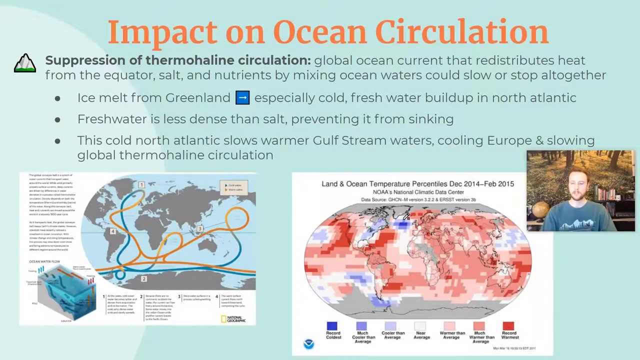 change it is a suppression of the thermohaline circulation and let's look at why we have this graph here of temperature anomaly at the surface from noaa and so what we're going to see is that almost everywhere on earth has been warming dramatically but what we have is this abnormally cold area up here in the north atlantic just south of greenland now this is due to melting ice that's already been completely melted this is because that's the way i say here in the north of greenland and so what we have is a very cold area crashed into the surface of the ice sheets and it's entering the surface water so what we're adding is really cold fresh water now this is a problem because that fresh water is less dense than the salt water so it's going to sit up here on the surface and so instead of sinking it's going to stay on the surface and it's going to do a couple things one of the things that it's going to do is it's going to distribute some of this cold into Gulf Stream normally brings warm air and distributes it to Europe. So Europe is much warmer than areas at a similar latitude that we would see, you know, in Canada or north of the US border here. And so that's a really critical component to Earth's or to Europe's, I should say, kind of microclimate or local climate. And so what this does is shuts off not only that Gulf Coast, because now as the Gulf Coast tries to come forward and move up into the North Atlantic here, it's running 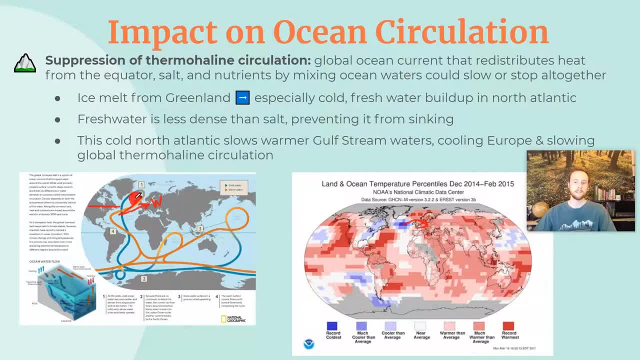 into this cold, less dense and fresh kind of mass of water that's coming off Greenland. And so that ice melts, it sends that mass of cold, fresh water that again, basically shuts off the thermal haline circulation. So this is a really big problem. Again, it can mean colder weather for Europe, but it can also mean that we stop cycling nutrients and oxygen and stop distributing heat 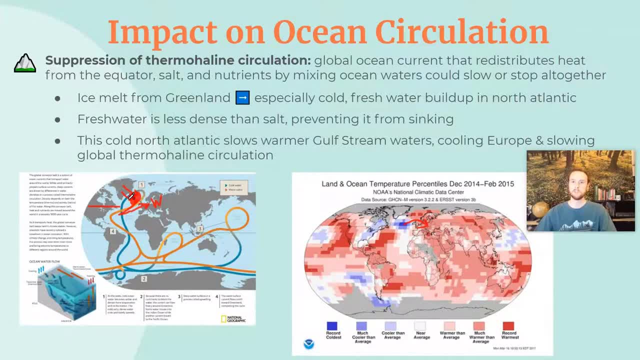 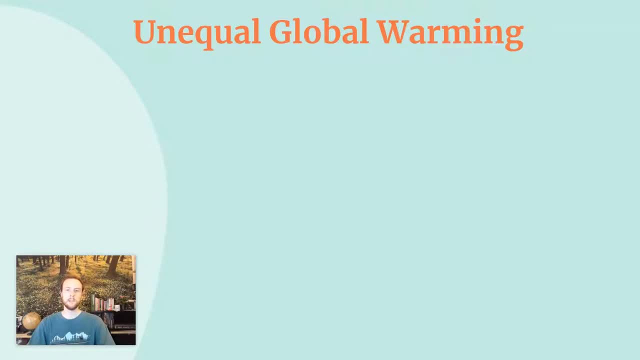 so evenly throughout Earth's surface and through the ocean. Next, we'll look at how climate change and specifically global warming have impacted the poles dramatically in a different way than the rest of the world. And so again, we need to know that the polar regions of Earth are warming faster than anywhere else on Earth. And this is due to a variety of different reasons. The overall concept 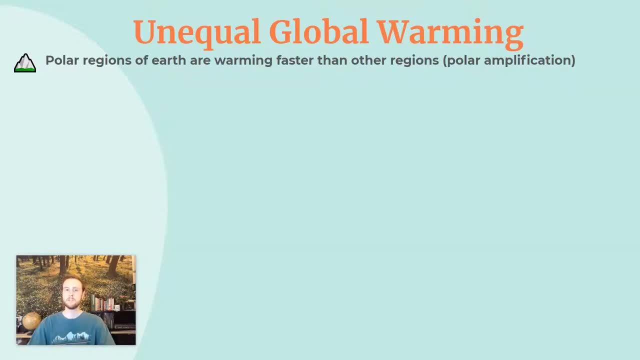 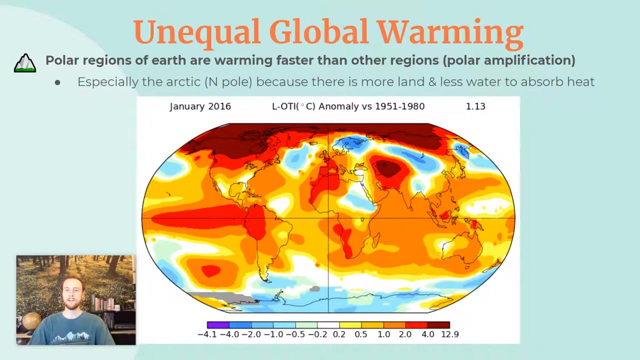 at play here is something called polar amplification. So that's an important term we should know that refers to this idea that poles have a pronounced, warming effect from Earth's climate warming. So the first region, or the first reason I should say that these regions are warming at a faster rate, and especially that the North Pole is warming at a faster rate is because there's just simply more land in the North. And land has a lower specific heat. Land does not absorb excess heat in the same way that water does. So if we look at this 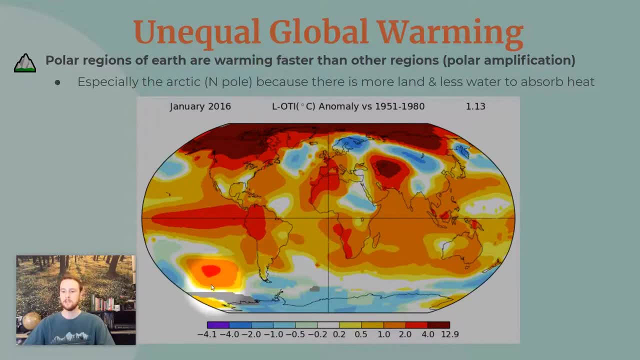 temperature anomaly map from NASA, what we can see is that in the Southern Hemisphere, we just have a lot more open ocean. Open ocean, because we have a lot more open ocean, we have a lot more 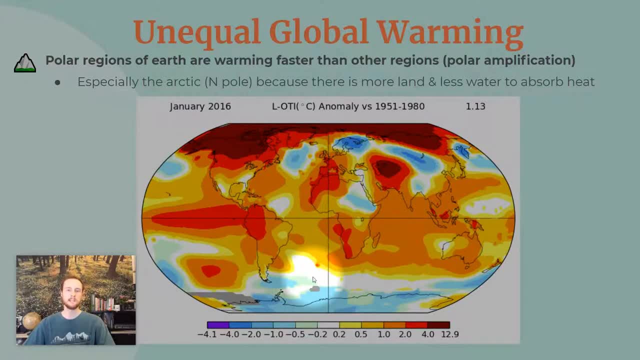 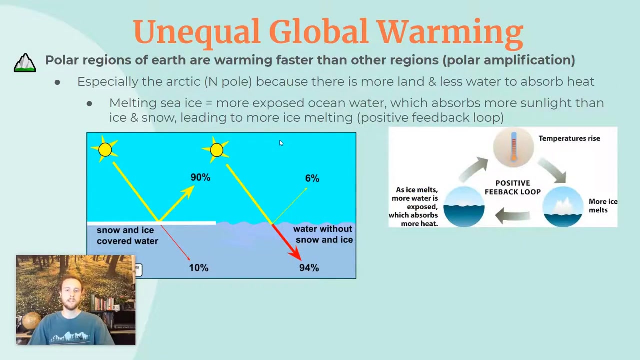 water has such a high specific heat, is really good at taking on excess heat and storing it and not transferring it to the ice sheets here. However, if we look at the Northern Hemisphere, we have far more of Earth's land concentrated in the Northern Hemisphere. Earth's land has a lower specific heat. And so, it does not absorb nearly as much heat the same way that the ocean does. So what it's going to do is transfer more of that heat to the ice in the North and that's going to lead to the polar regions warming faster, but also to the ice. So that's what we're than the South Pole regions now if we look at another reason here it's albedo so remember that ice and snow have very high albedo or reflectivity meaning that they bounce a lot of the incoming insulation right back out of Earth's atmosphere whereas water is a pretty dark deep blue color and so open ocean is going to absorb a lot more heat and so what happens is a positive feedback loop as the climate warms it melts sea ice that exposes more open ocean to the sun's rays which in turn absorbs more sunlight and generates more heat it gives off that heat and it melts more ice nearby and again we have a vicious cycle which we call in science a positive feedback loop and so we have 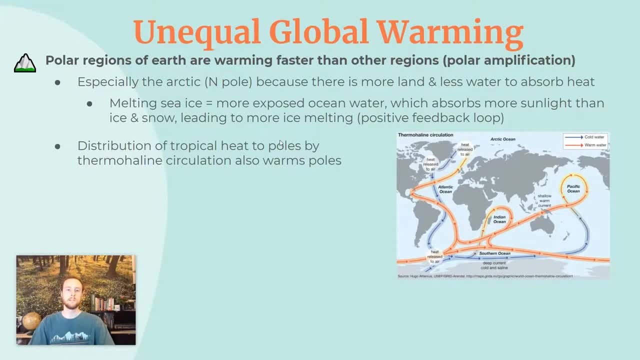 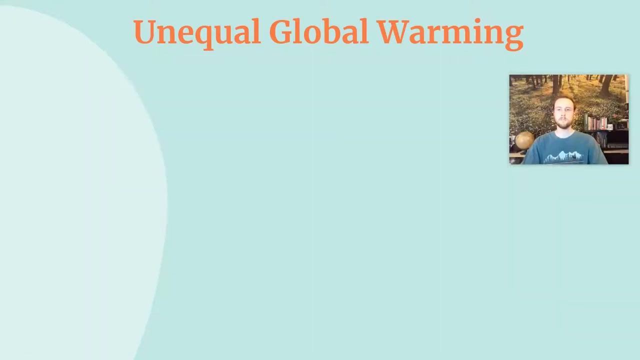 one more reason here that the poles are being impacted disproportionately from the rest of the earth and that is the thermal haline circulation so remember that a lot of this heat generated in the ocean is going to be generated by the water at the equator and generated at the subtropical regions it's going to be transferred out and so because we have that warm surface water that's flowing away from the equator moving towards the pole that water takes this warmth out away from the equator and redistributes it to the poles by transferring it to the air in those polar regions and so both the North and South Pole experience a lot of the heat that comes from equatorial and tropical regions heading out their way and it basically contributes to a third reason that we have this polar vacation or this increased warming of the poles we talked about the positive feedback Loop when it comes to the albedo of polar regions and decreasing polar ice increasing ocean that's exposed but remember there's also the positive feedback Loop with respect to the permafrost and with respect to methane 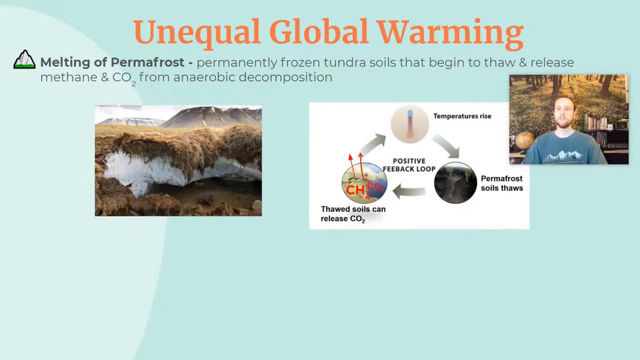 so this was covered in part one this is repeat information you don't need to write this down if you're taking notes but I just wanted to hear as a reminder 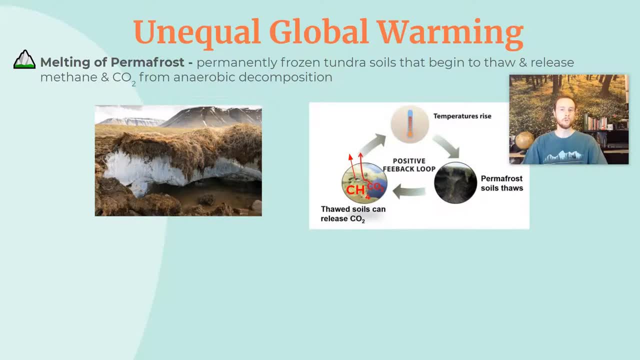 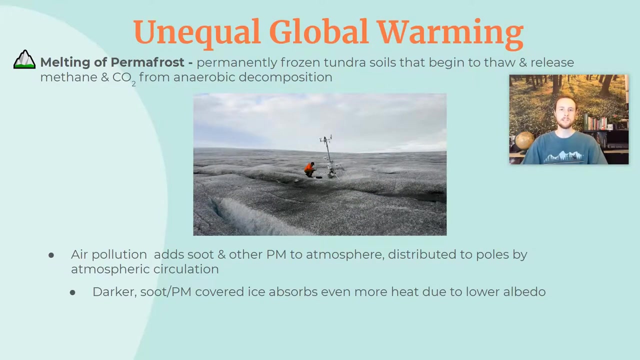 another issue that kind of exacerbates or worsens this positive feedback Loop is air pollution so we have particulate matter specifically things like soot or little black particles that are going to be distributed by Earth's global atmospheric circulation is going to end up out at the poles what happens is that soot that particulate matter falls onto ice and it's going to lower the albedo of ice it's going to make it darker and it's going to make it absorb more heat so this is just another reason that the poles are experiencing especially pronounced warming when compared to other regions the ice that normally cools them that normally reflects sunlight is not only being melted due to increased temperature but it's also being melted due to a decreased albedo or decreased reflectivity based on this air pollution and then finally we'll look specifically at polar ecosystems 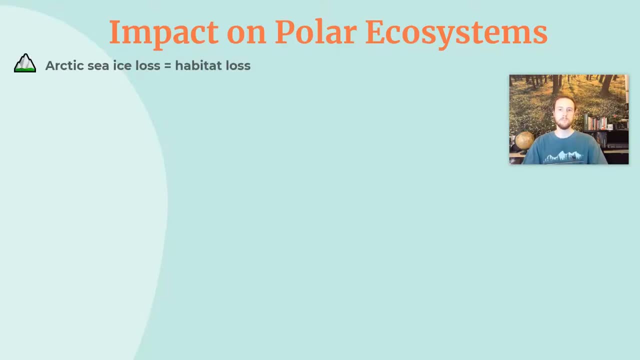 and so the loss of Arctic ice is going to mean that we're losing habitats we're losing areas that organisms need to live to find food and to rest when they're swimming and so we have